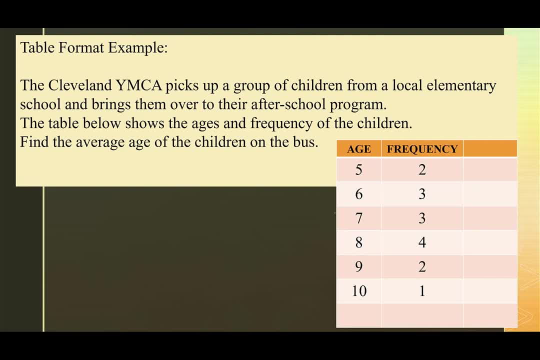 8 plus 9 plus 10 together and find the average of those 6 numbers, because there's more than 6 kids on the bus. So how many kids are riding this bus? I want you to add this frequency column and that gives you a total of 15 kids. 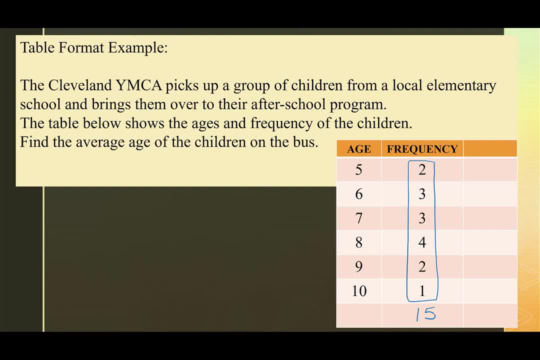 Next to find the average age, we could take the long route and add each of these 15 ages together. For example, 2 children were 5 years old, so we could say 5 plus 5.. 3 children are 6 years old, so 6 plus 6 plus 6.. 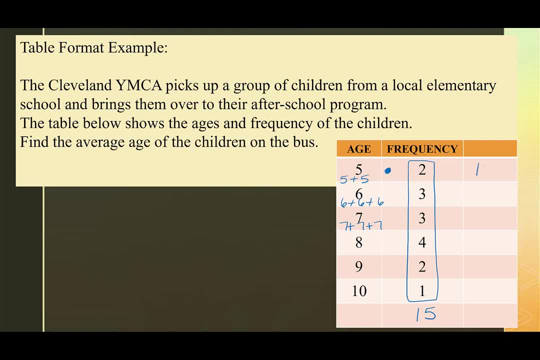 3 children are 7 years old, so 7 plus 7 plus 7.. 18, 3 children are 7, 21,. 4 children are 8,, which is 32,. 2 children are 9,, which is 18,. 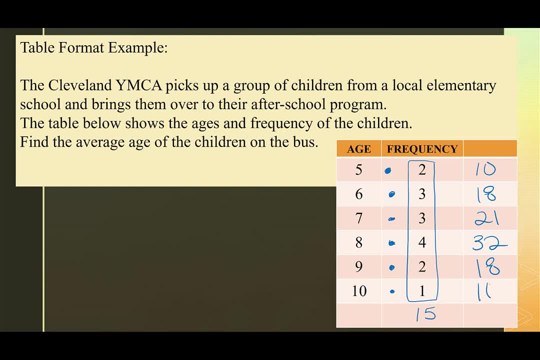 and 1 child on the bus is 10,, so 1 times 10 is 10.. It's much easier to add these values together because there's only 6 of them. Go ahead and add these numbers together on your calculator and I'll do the same. 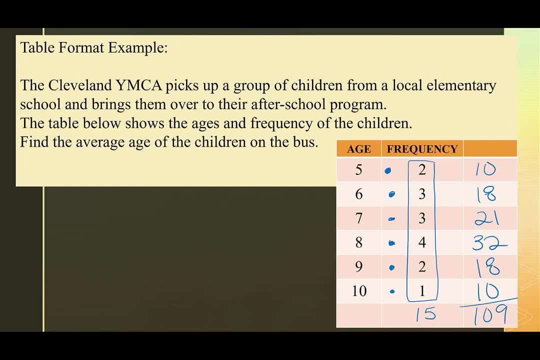 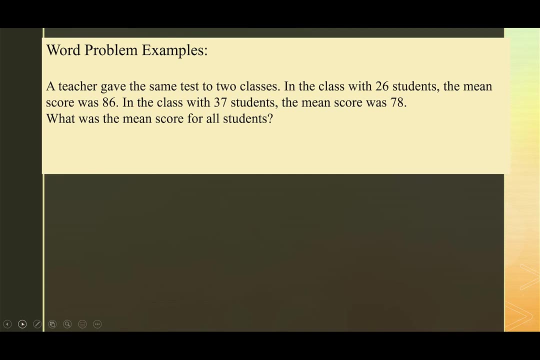 You should have a total of 109, and then we'll take the total 109 and divide by 15, and so the average age is 7.27.. Next, this example is finding the mean with just using a word problem. A teacher gave the same test to two classes. 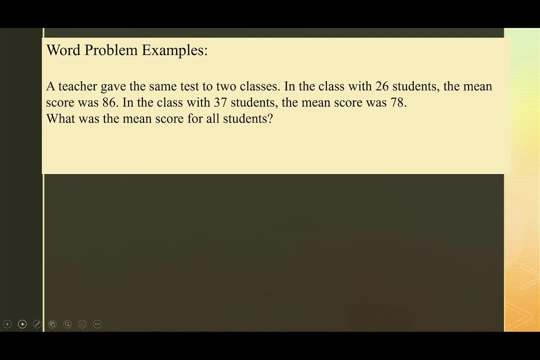 In the class with 26 students, the mean score was 86.. In the class with 37 students, the mean score was 78.. What was the mean score for all? The first question I want you to figure out is how many students. 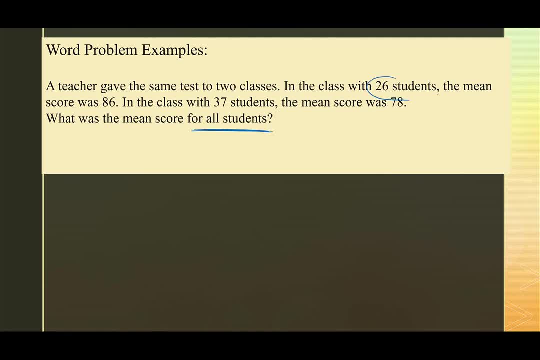 What does it mean when it says all students? Her first class had 26 students, Her second class had 37, so 26 plus 37 is a total of 63 students. To find the average we need to know the total of all 63 exam grades. 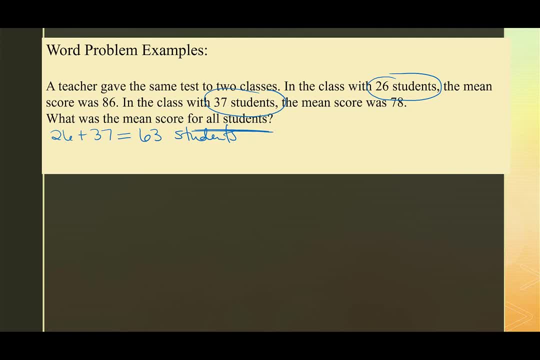 Well, we don't have that information specifically, but we do have other information In the word problem that can help us. Let's look at this one class at a time. Take a look at the information we have for class number one. 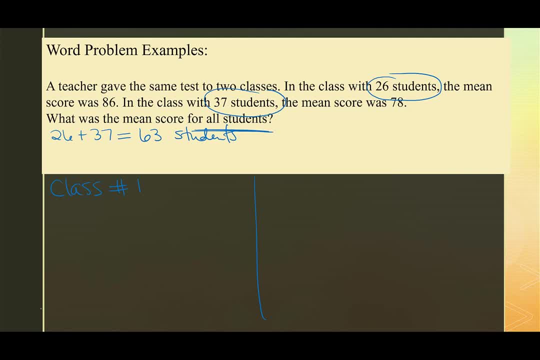 In the class with 26 students, the mean score is 86. So we can set up the equation: X over 26 equals 86, and we're going to let X equal the total scores of class number one. So if we have a total scores of X, 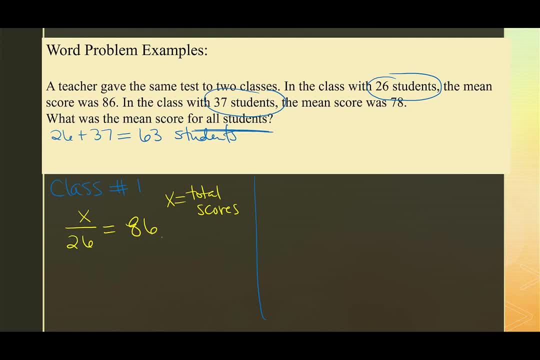 When we divide by 26.. 26, we know the answer is 86, because that's the information given to us in this word problem. Now I want you just to solve this equation. In order to get x, we're going to multiply. 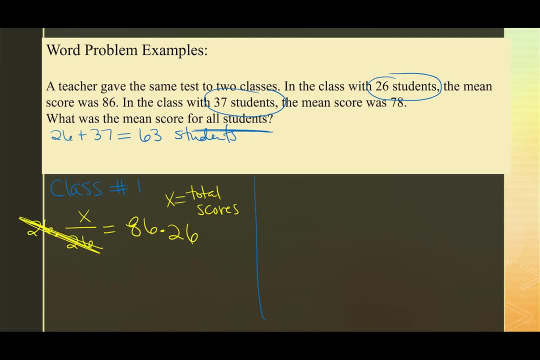 both sides by 26.. These 26 on the left side cancel Multiply 86 by 26, and x equals 2236.. That is the sum of all 26 exam grades for class number 1.. Next let's look at class. 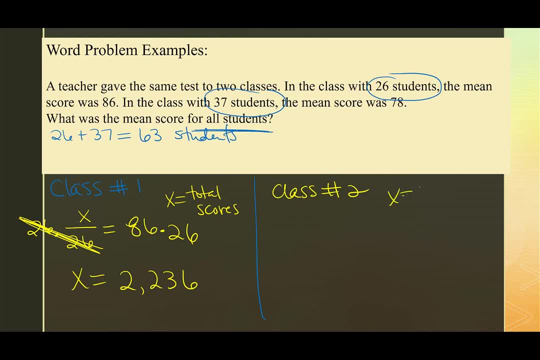 number 2, and we're going to go through the same process. We're going to let x be the total scores. x divided by 37 equals 78.. We'll multiply both sides by 37.. x equals 2886.. One more step Now. I want you to combine the total scores from class 1 with the total scores. 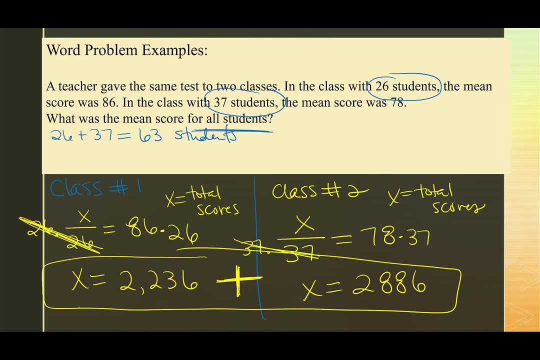 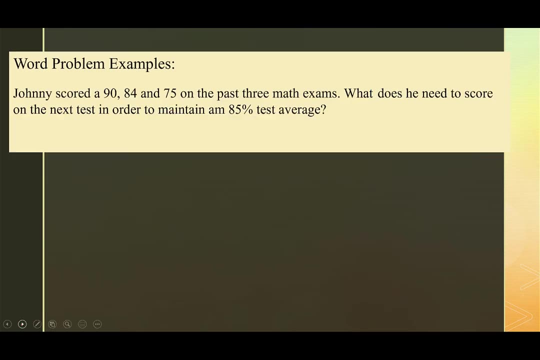 from class 2.. By adding these x values together- and I've ran out of room, So up here- the total score is 5122.. Let's divide that by 63 students for a mean score of 81.3.. The next example. 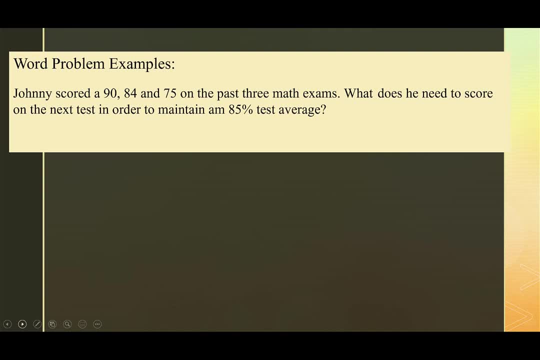 Johnny scored a 90,, 84, and 75 on the past three math exams. What does he need to score on the next test? in order to maintain an 85 test score? He needs to score on the test average. So we're going to use what we know about the 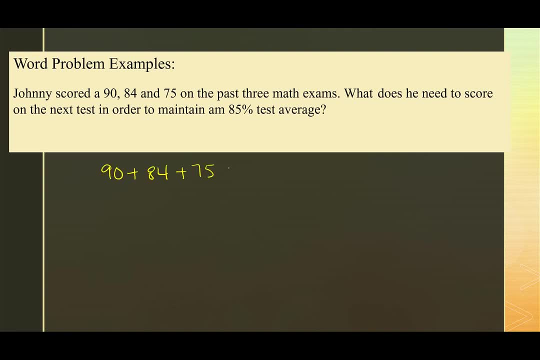 mean and set up another equation. We know that we can add his four test scores together, even though we don't know what that fourth test is. I'm going to call it x, for right now We know, when we add those together, divide by 4, that Johnny wants it to be an average. 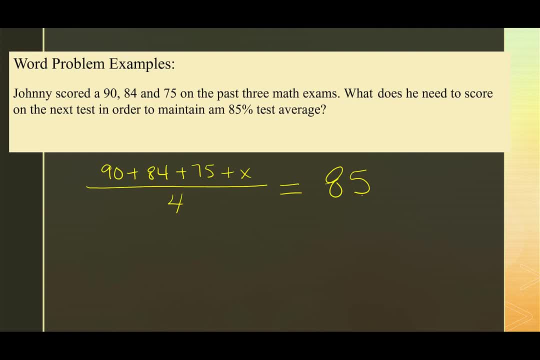 of 85.. So we're going to just take this equation and solve for x. The first thing I want you to do is add the three test scores together. This is 249 plus x, And then we're going to divide by 4 equals 85. And it times 4 to both sides: 249 plus x equals 340.. And then 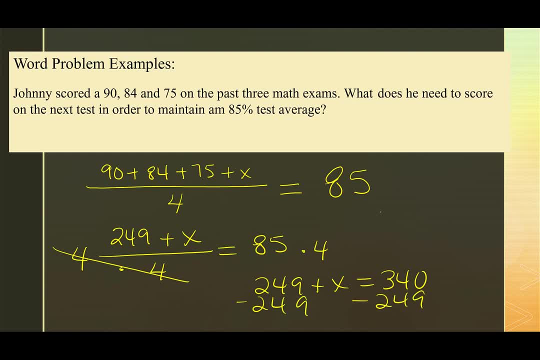 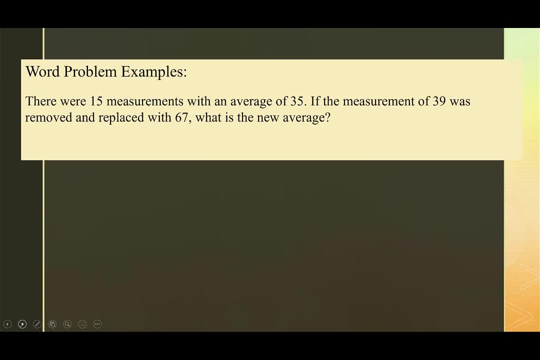 you subtract 249 from both sides And that fourth test, Johnny needs to make a 91% to maintain an 85% test average. Here's another word problem. There were 15 measurements with an average of 35. If the measurement of 39 was removed and replaced with 67, what would? 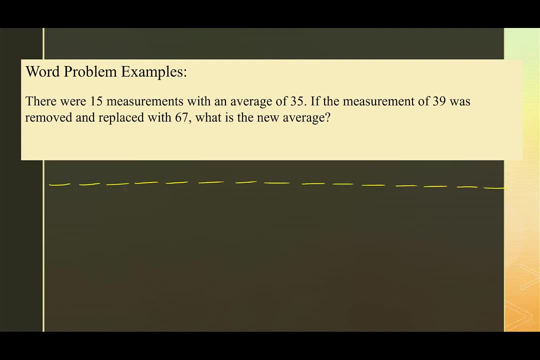 happen. What is the new average? Okay, so I have 15 lines across the screen. that represents the 15 data points. We don't know the individual data points, but we do know when we add them all together and we'll let x be that total when we add them together and divide by 15,. 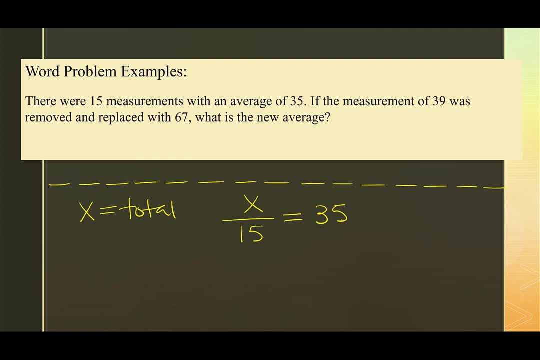 we get an average of 35. So by solving for x we can find out what the total measurements were. I want you to multiply 15 to both sides. 35 times 15 equals 35. And then we're going to subtract 39 to get a total of 525.. So in the original 15 measurements, when you add: 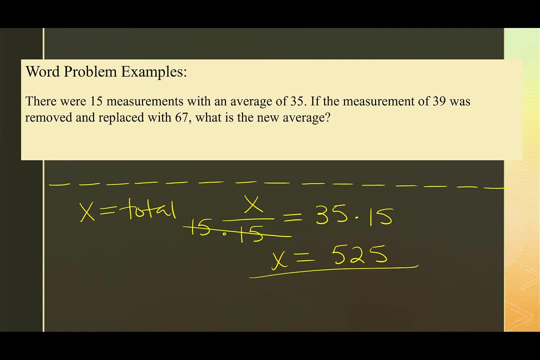 each of those 15 measurements. together you have a total of 525.. Now the question: something is about to happen. You're going to remove the measurement 39, it's a single measurement. 39 was removed- and replace it with 67.. So, on the left-hand side of the screen, I want. 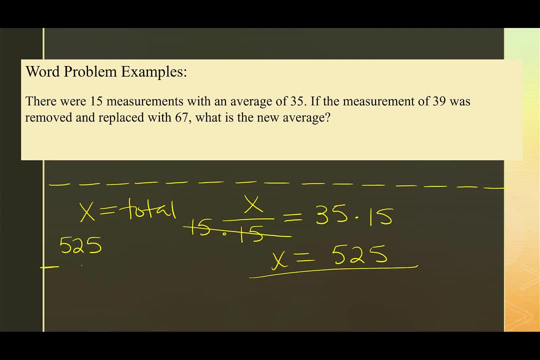 you to follow this math, I'm going to do 525.. I'm going to subtract 39 to get a total of 486, and then add the new measurement of 67, and that is 553.. So let me walk you back. 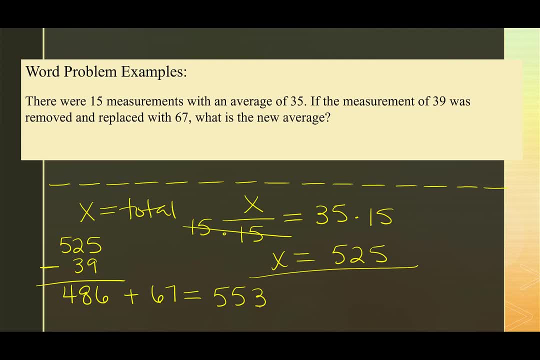 through that again. If we know, the original 15 measurements had an average of 35, that means the original 15 measurements had a sum total of 525.. If we took one of those measurements, specifically the measurement of 39, we took that out and replaced it with a new measurement.